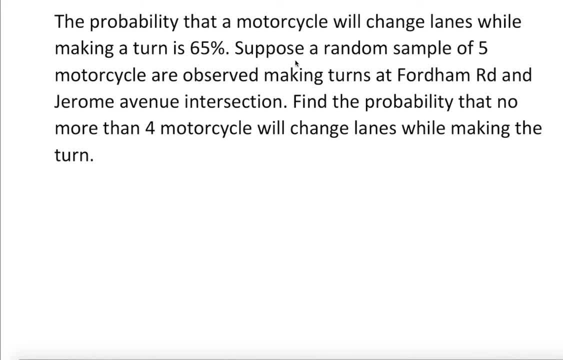 Motorcycle will change lane while making a turn is 65%. Suppose a random sample of five motorcycles are observed making a turn at Fordham Road. in Jerome Avenue intersection, I find the probability that no more than four motorcycles will change lane while making the turn. So I'm going to use a binomial probability distribution table. We can use calculator, We can work it out by using the binomial formula, But this time I'm going to show how to use the binomial distribution table. 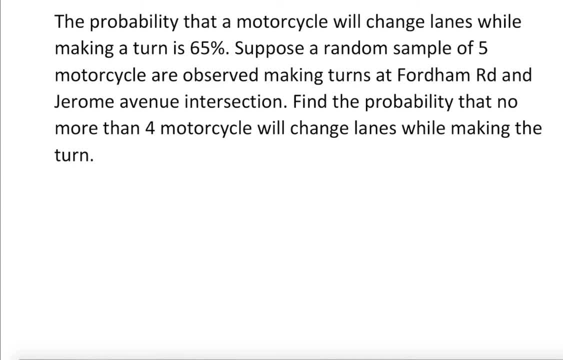 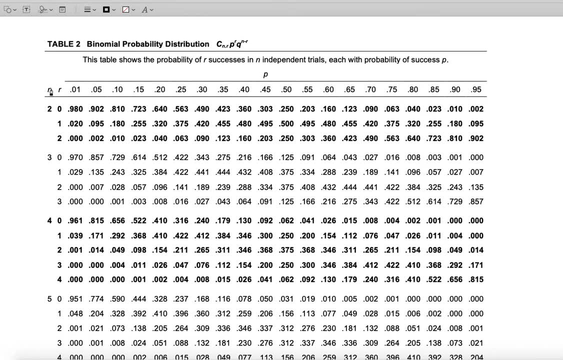 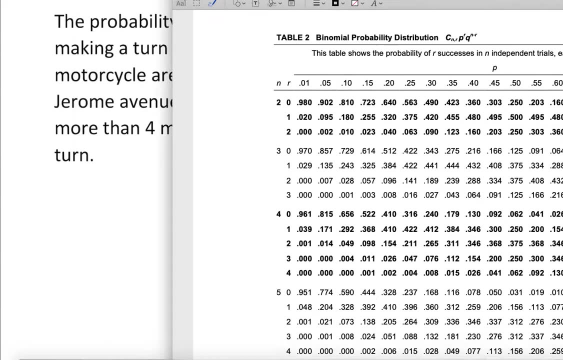 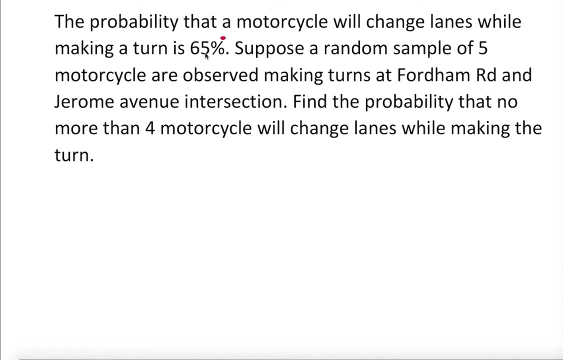 Which is the easy way of doing. Well, before we use, what is the binomial distribution table? So this is the binomial distribution table. As you see, it has this is the formula- And it has n. Sometimes you have x and the p. So these three things we have to know, We have to identify these three things. Okay, So 65%? Let's take a look here. What are the information? So 65%, that's the p, That's p And this is a fixed trial. 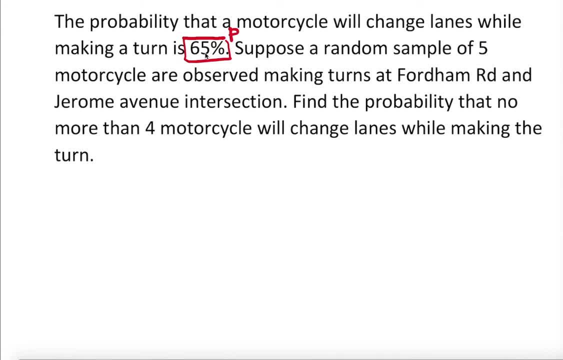 So that's the n. Well, I'm going to put down here: That's the n. So this is going to be my n Fixed number of trial, And this no more than four bicycles. So seems like this one is telling us we cannot exceed four. Okay, We cannot exceed four. So that would be my x, or that would be my r, Small letter x or small letter r. So once we know this, 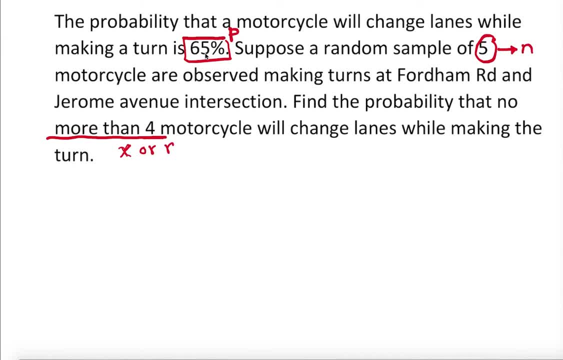 we can actually pull out the information Actually. well, use the formula table. So, as you see, n is a fixed trial, n is a fixed trial, So the n is equal to five. And of course we know the p, which is 65%. So we know this p is 65%, So this one is no more than four motorcycles. So I want to check out here something very clearly. So we have a trial, How many trial? One, two, three, four. 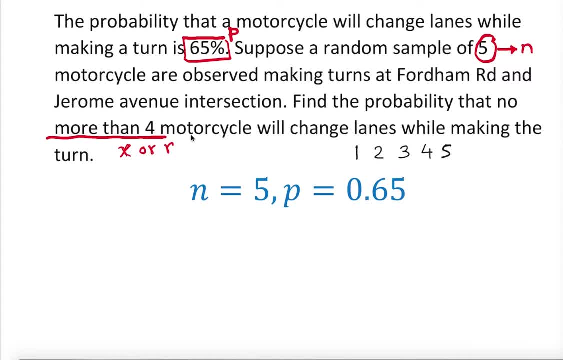 Five trial. Remember, that's the five maximum trial going on. Okay, So they're saying that I cannot go over no more than four. No more than four. So that is basically. well, actually that should be zero here also. Okay, So this is the number of trial we look into here. So well, we can come up with basically. 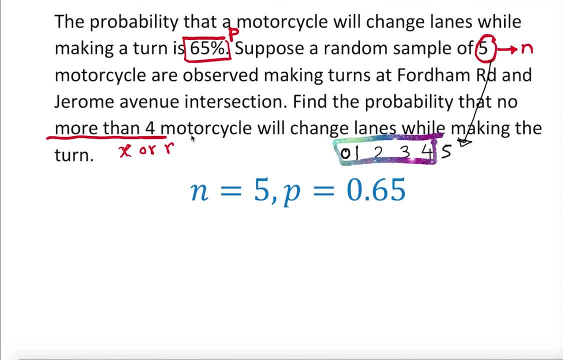 at least. well, so I'm sorry- more than four. So probability of no more than four is equal to x, less than or equal to four. Why is x less than or equal to four? Because they said no more than four We cannot exceed, We cannot include five here. So it's basically all of this: Zero plus one plus two plus three plus four, Not those numbers, the probability we're going to add. So 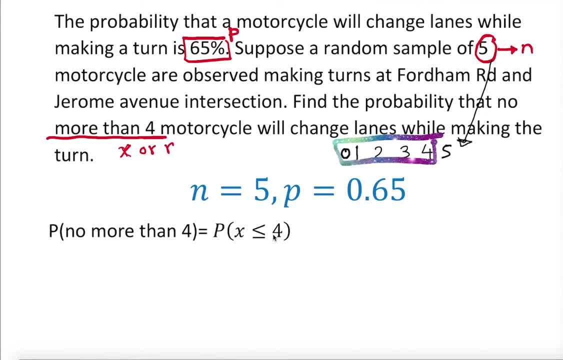 this is x less than or equal to four, So the x value must be on the left side, or whatever entries. So is equal to, I can say, probability of zero plus probability of one, plus probability of two plus probability of three plus probability of four. Then we are ready to go check it out, Our binomial formula: plus x equal to one, plus x equal to two, plus x equal to three, plus x equal to four. 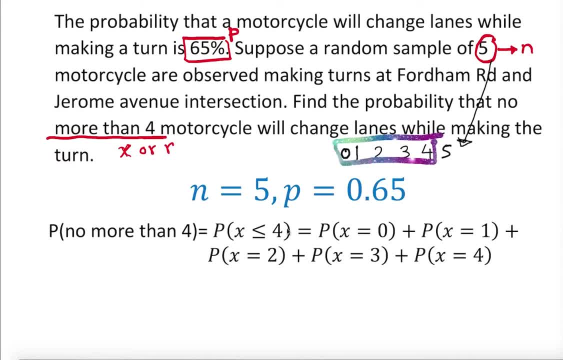 This is what probability of x less than or equal to four, or no more than four, No more than four. So that's what that's how we actually expand it, Coming from here actually. So we are one, two, three, four, So one including zero. One, two, three, four. Okay, Now we can go to the binomial probability distribution table. So how we do that? Go to n, which is a five. 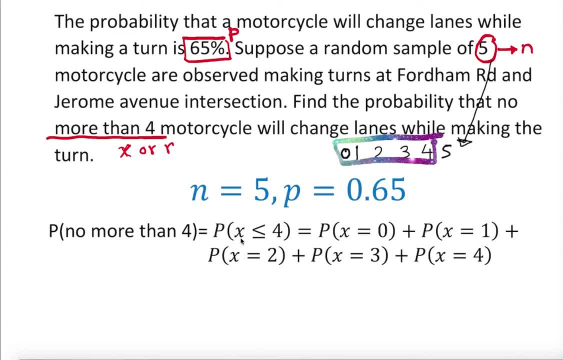 x is the probability 65. And that is going to be the x or r, depending on which book has what kind of formulas set up. Some book has a r as a specific number of success in an n trial, Or x is a specific number of success in n trial And phi stands for probability of a success in n trial And obviously n is the fixed trial. So let's go ahead and do that. 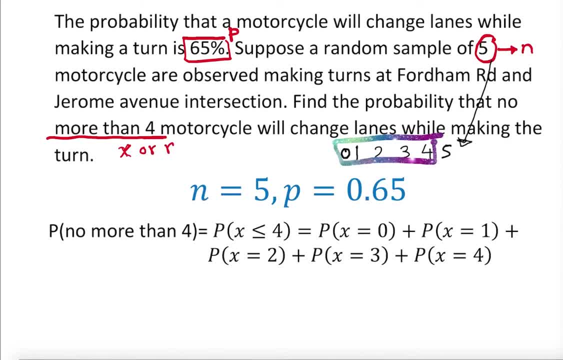 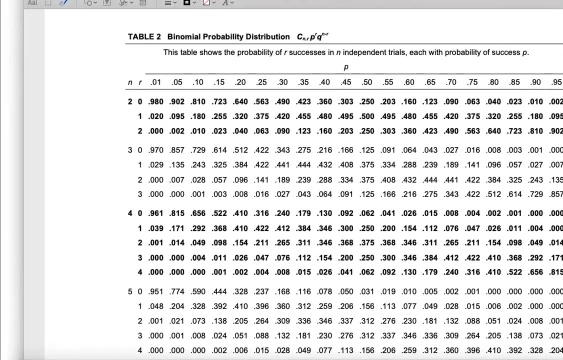 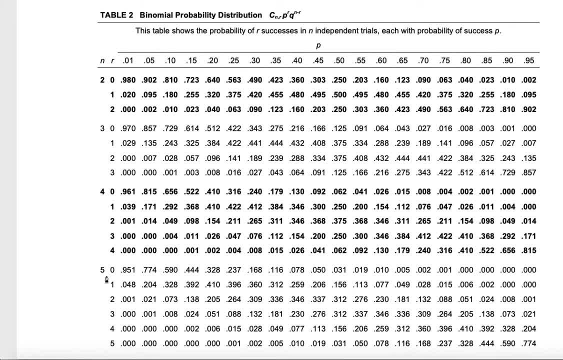 if you look into n is 5, here you go. so that's the n is 5 and this one represent to the right side. if n is 5, we have 5 maximum, including 0. so this is x or r, it doesn't matter what is given. so 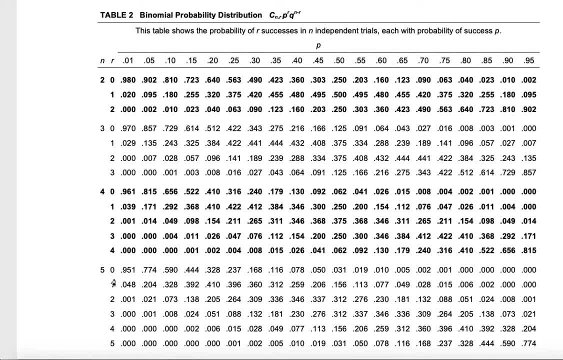 you look into that now. we can go with 0 all the way to 4. so, but where should we stop? look, there's so many numbers are there. so we go this row here. this row here is basically for probability. so our probability in this case is 65. so we are lucky, we have a 65 probability. 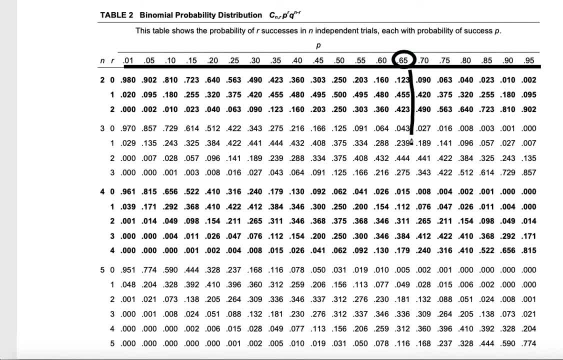 so then, what we do? we go down here and obviously we go 4 and just get all those. this is basically what we have, we should have. well, i'm gonna have to move it, so this is gonna be one. that's it, so this is the probability we are going to need. so, again, how to do that? we go n, which is: 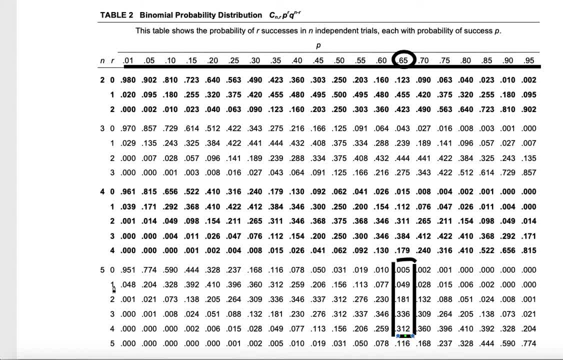 the 5, and of course, then x is a limited. we're going to go 0- 1. we add all of this actually after including 5. why? because we cannot go more than 4. they said no more than 4, so that's what it is. 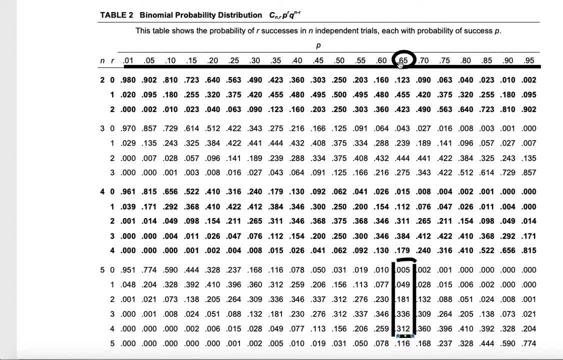 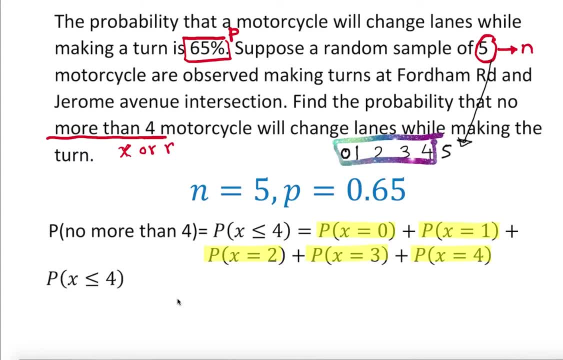 and we come off here under 0.65 because that's the p. okay, so we have everything ready less than zero. we clearly see all of this and we take any calculator, this should give us approximately 0.883. we can do a little bit different oils. we can do a little bit different oil. what is that? we basically 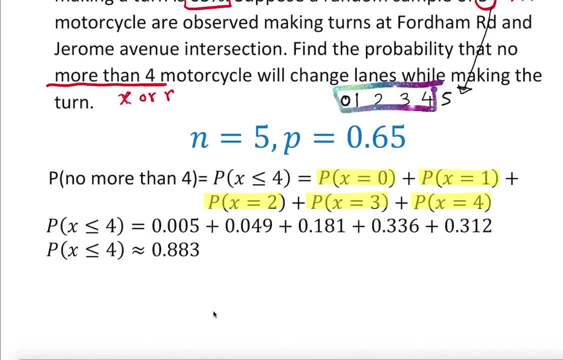 use the at least concept. so what is at least concept? at least concept is: probability of no more than 1 is same as probability of r less than equal to 1 or 1 minus probability of x equal to 5, because the probability of x is. 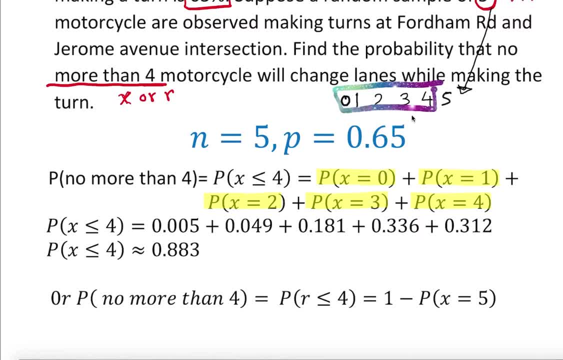 because we know everything, just only one thing. look at this here. so if we can somehow, we know total is going to be one- if we can somehow subtract this last one, we can get answer clearly. so we don't have to do all this, we can just use this concept here. so if you use this, 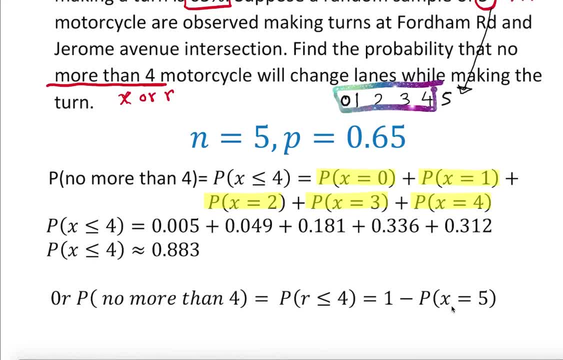 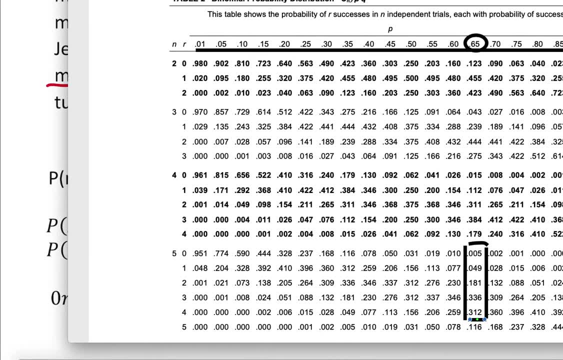 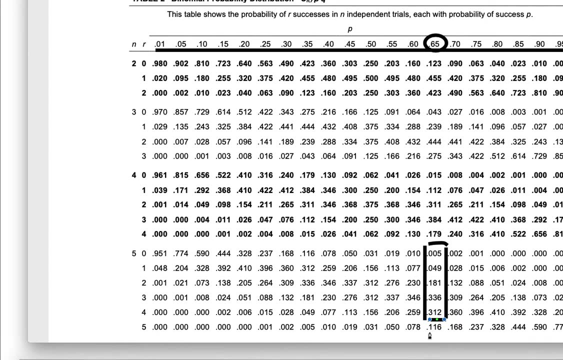 concept here: probability of one minus probability of x equal to five. so what is probability of x equal to five? let's do this here. so in this case, we're looking for x equal to five. in other word, we go under 65, we go under 65 and we look into x equal to five, which is 0.116, 0.116. this is the 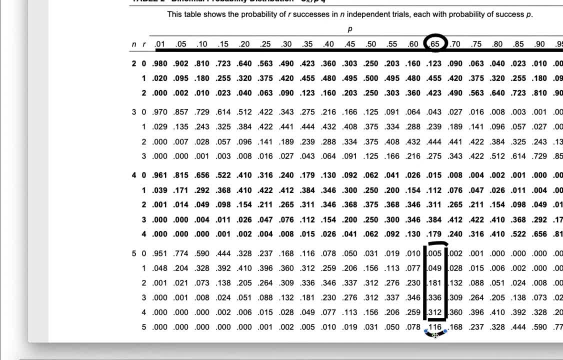 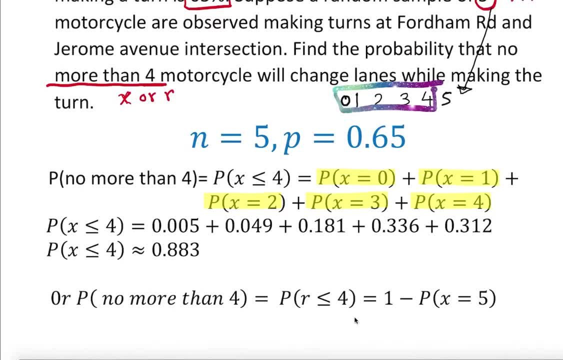 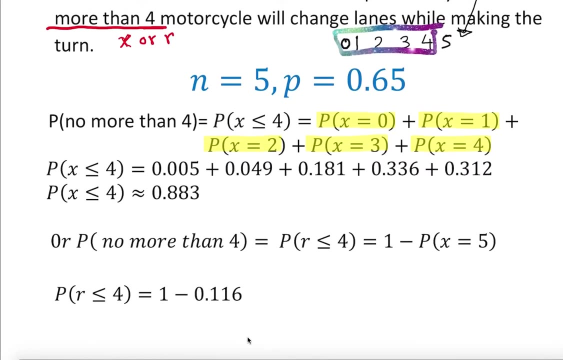 one. we are interested now, this time 0.116, 0.116, and we're going to subtract this one from one, which is very same thing actually. so, so, so, so we basically have to subtract one minus probability of five, and once we do that, we get the same thing. well, clearly, you see a little bit of because of 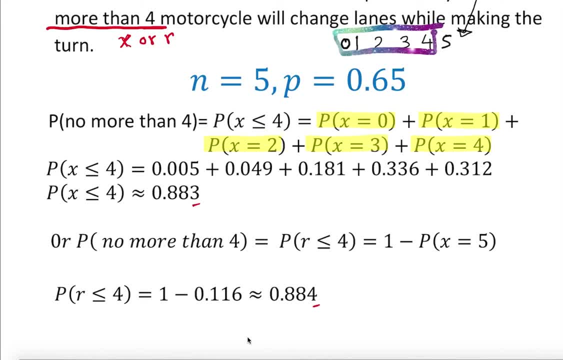 roundup actually, otherwise it's basically the same thing. so we can do both ways, the top way or on the bottom way, but again, if you know at least. if you know at least means you can do that. also one minus probability of at least one, which is, in this case, probability. 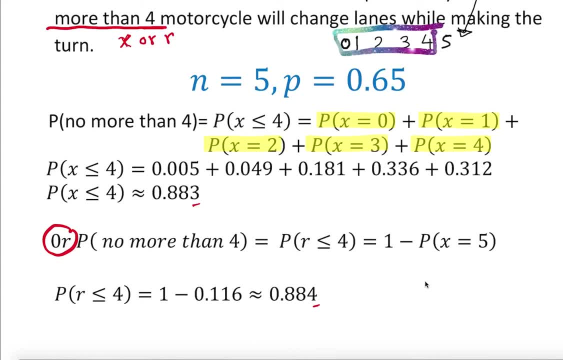 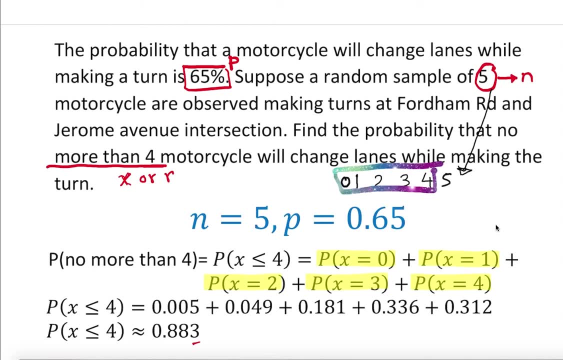 of x equal to five. that's how we use binomial distribution table and that's how we full out the information from our problem and find the probability.